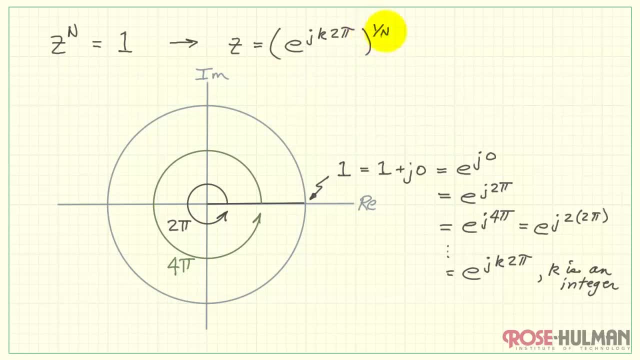 let me go ahead and substitute that back in here And I'll bring the exponent inside the parentheses. Now, here we have a series of values for z. We have z raised to the nth power. therefore we need n roots And I'll have k run from 0,. 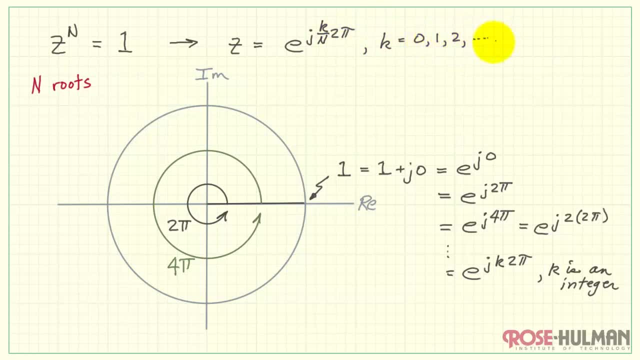 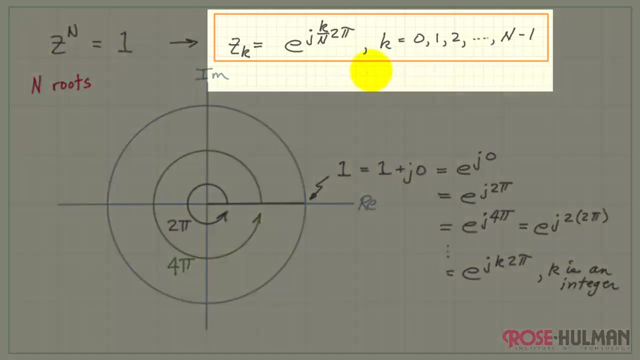 1, 2, all the way out to n minus 1.. All together, we have n values of z. Each of these values is a root, And this gives us the finished equation for the nth roots of unity. Let's visualize these roots in the complex plane. 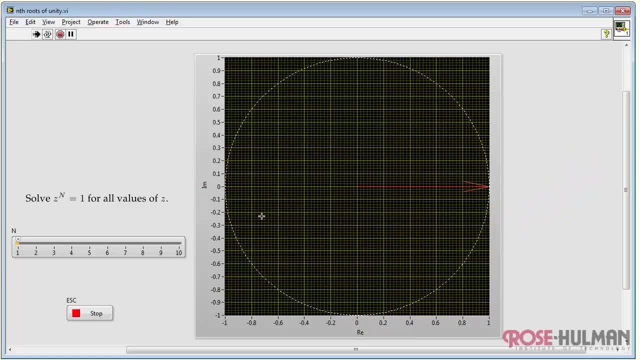 For a variety of values of n. I'm picturing the complex plane. Here's the solution: for n equals 1.. For n equals 2, we have two solutions: negative 1 and positive 1.. For n equals 3, we see that we have one root at 1, but the other two roots have complex values. 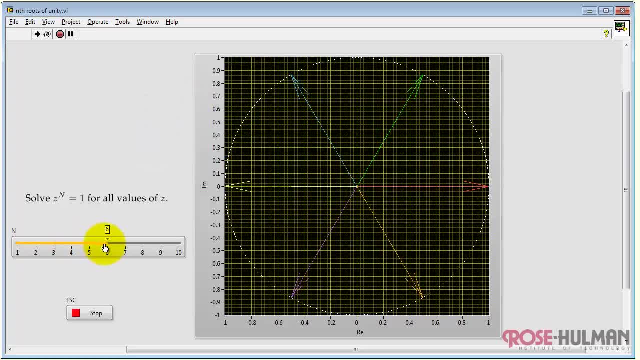 Altogether, we see that we have n roots at 1, but the other two roots have complex values, And so we'll see that the roots are arranged in such a way that we have n equal sized wedges. Note that positive 1 is always a root. 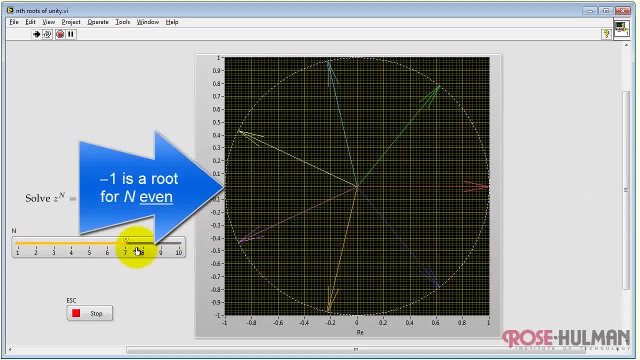 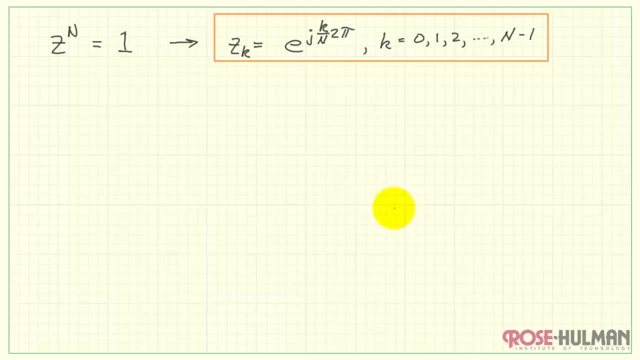 Negative 1 is sometimes a root, And in fact it's a root only when n is an even value, as we can see here. All right, That gives you a visual picture of what these roots look like. Let's turn now to a related case of z to the nth power equals negative one. 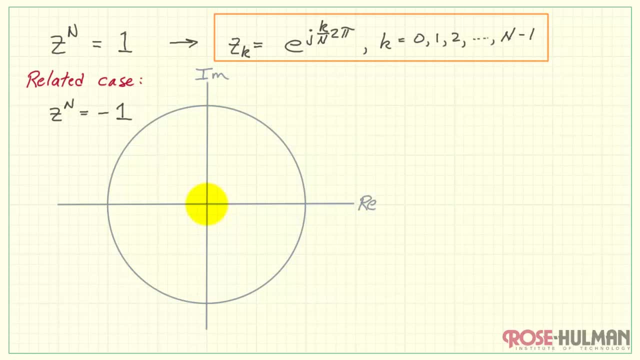 Let's take a look at how we might be able to deal with this negative sign. Returning to the complex plane, negative one would be a vector pointing from the origin out by an angle of pi radians. This is equivalent to the angle minus pi radians and for this development, the